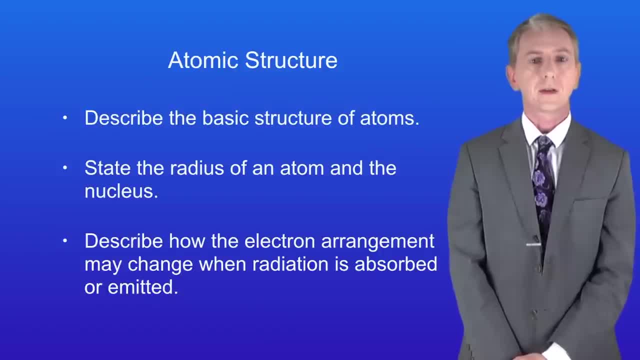 arrangement may change when radiation is absorbed or emitted. Now I should point out that this topic does overlap with chemistry, so if you've already watched my chemistry videos, then a lot of this will be familiar. However, there are some details specific to physics, so you still need to make sure that you learn this. Ok, let's start by looking at the basic structure. 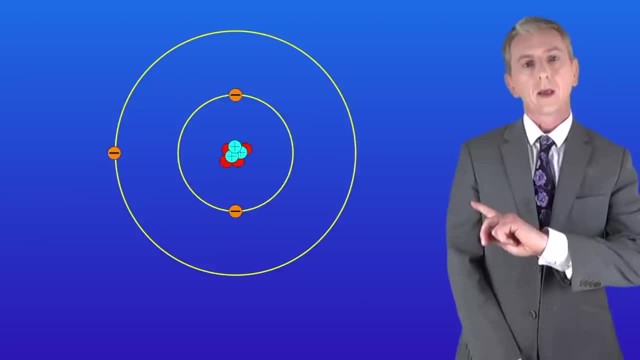 of an atom. I'm showing you a picture of an atom here Now. the first thing to notice is that atoms are very small. They've got a radius of around 1 times 10 to the power of minus 10 metres, and you need to learn that Now, this is an approximate figure, as some atoms 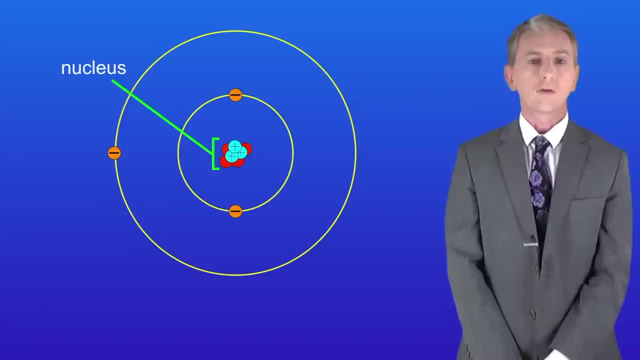 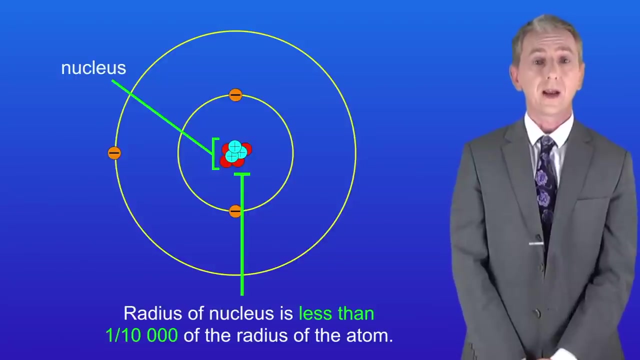 are larger than others. Atoms contain a central region called the nucleus, and the radius of the nucleus is less than 1 ten thousandth the radius of the atom. In other words, the nucleus is tiny compared with the atom. However, almost all of the mass of the atom is concentrated in the nucleus. 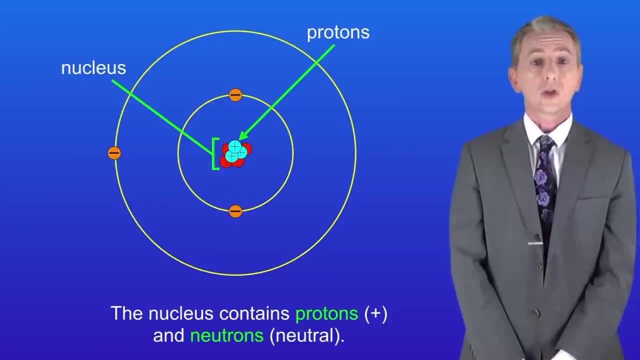 So let's look at that in more detail. The nucleus contains two particles. These are protons, which have got a positive charge, and neutrons, which have got no charge. they're neutral. So what that means is that the nucleus contains a small number of particles and neutrons which 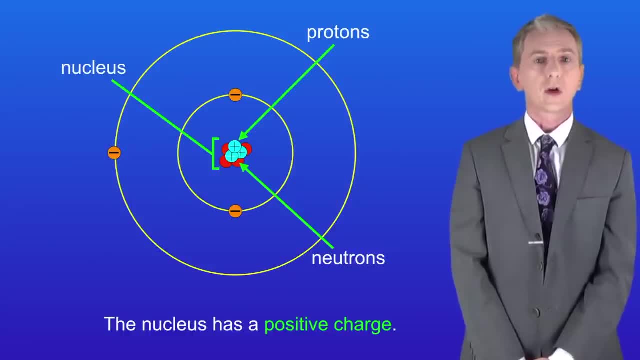 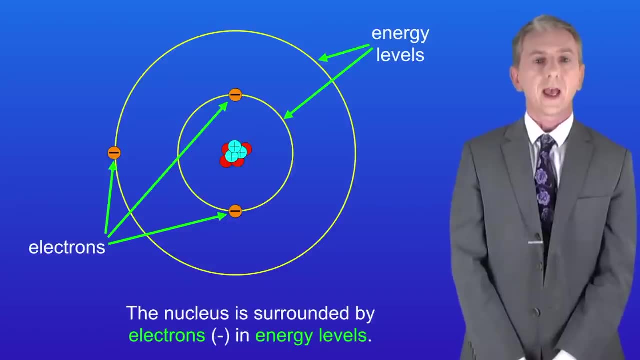 have got a negative charge. So we can see that the nucleus has an overall positive charge and that's due to the protons. Now the nucleus is surrounded by electrons and these have got a negative charge. We find electrons in energy levels, and energy levels are at different. 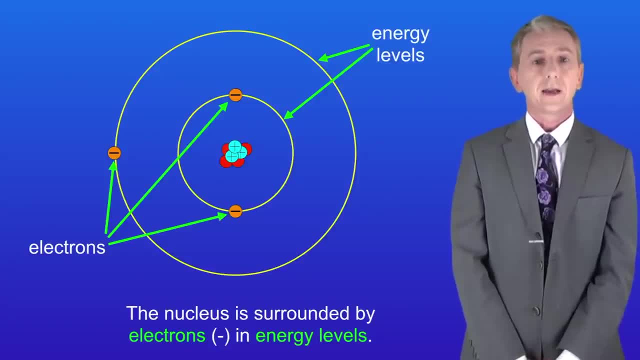 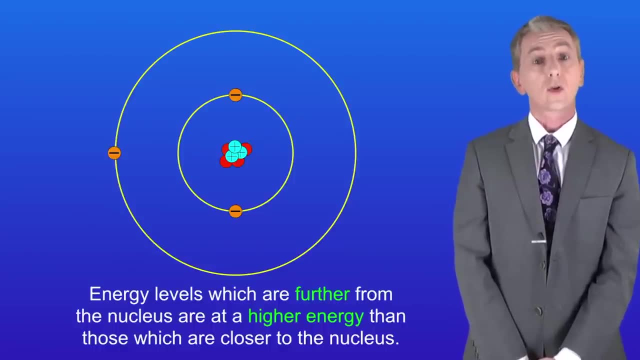 distances from the nucleus. Now there is one key idea about energy levels that you do need to understand: Energy levels which are further from the nucleus are at a higher energy than those which are closer to the nucleus, So this energy level is at a relatively low energy. 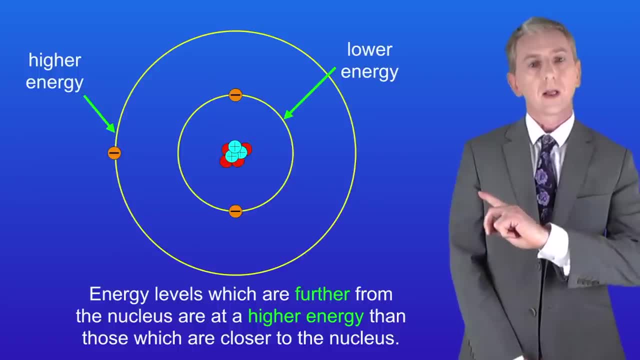 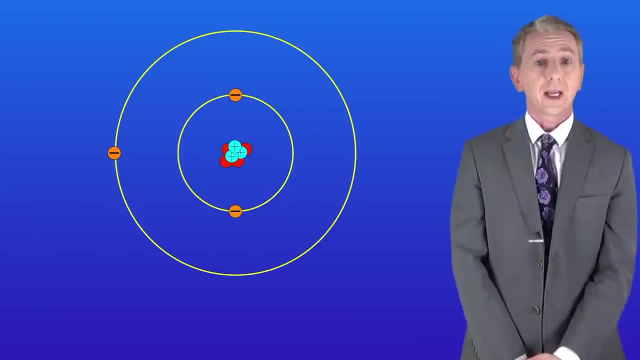 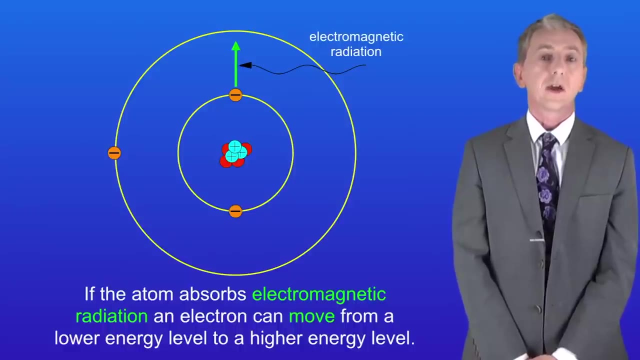 as it's closer to the nucleus, whereas this energy level is at a relatively higher energy, and that's because it's further from the nucleus. Now, electrons can change energy levels if they gain or lose energy, and we're going to look at that now. If the atom absorbs electromagnetic radiation, for example light, an electron can move from. 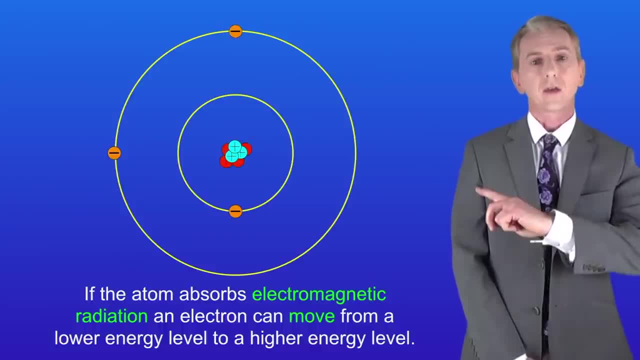 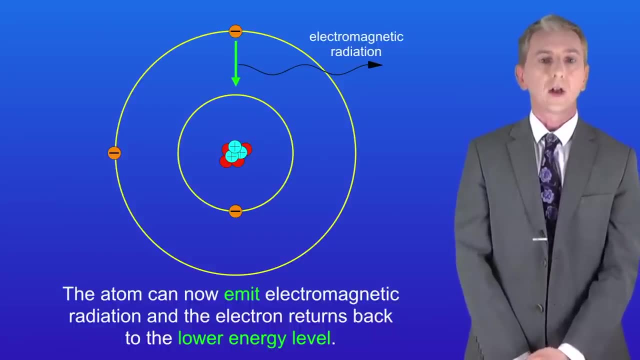 a lower energy level to a higher energy level, like this. Now, the atom can now emit electromagnetic radiation and the electron returns back to the lower energy level, like this. So, as you can see, by absorbing or emitting electromagnetic radiation, electrons can change energy levels. 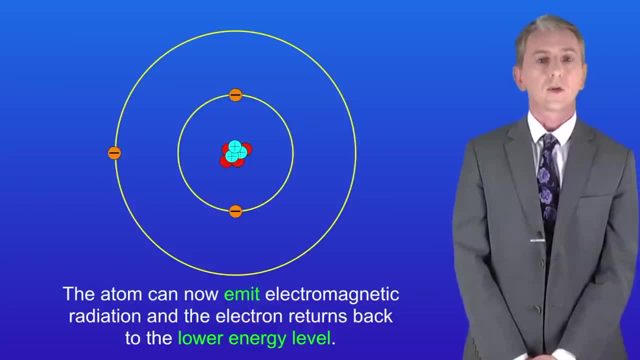 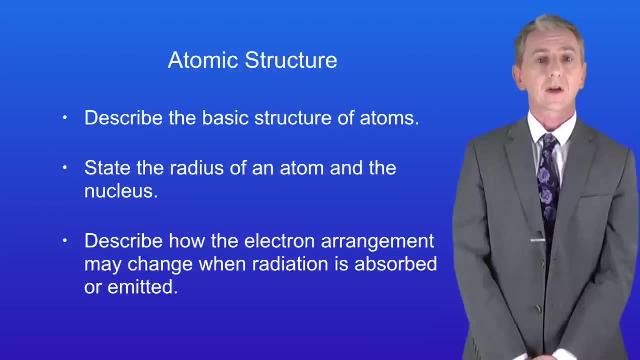 Remember, you'll find plenty of questions on the structure of atoms in my revision workbook, and you can get that by clicking on the link above. Okay, so hopefully now you should be able to describe the basic structure of atoms. You should then be able to state the radius of an atom and the nucleus. 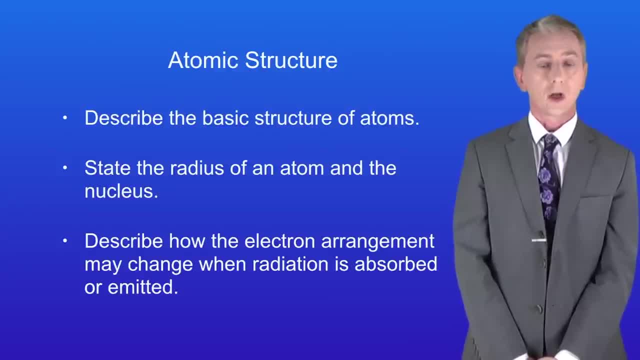 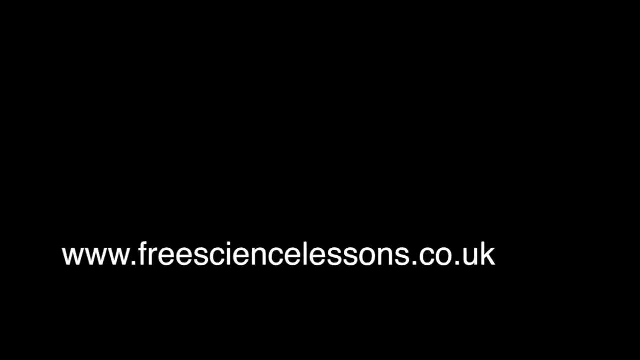 And finally, you should be able to describe how the electron arrangement may change when radiation is absorbed or emitted. 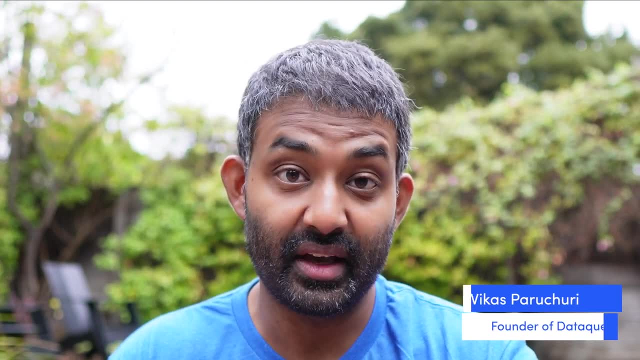 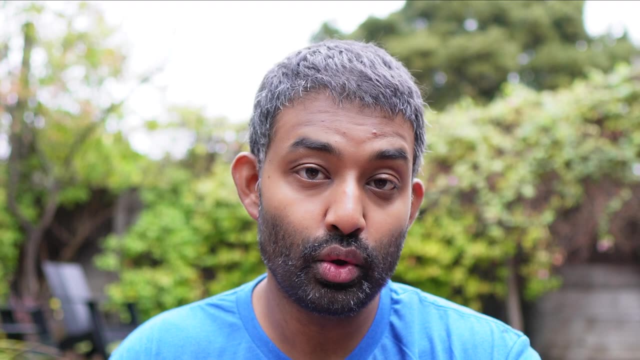 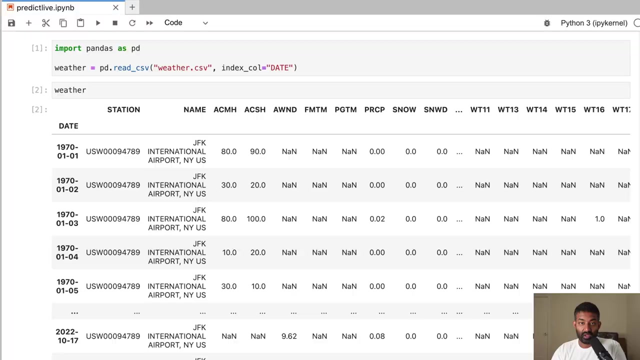 Hi, Today we're going to learn how to predict tomorrow's weather using historical data, Like: if it's raining today, maybe that means it'll be cooler than usual tomorrow. We'll be using machine learning and Python to make our predictions. First, we'll download our weather dataset, And the great thing about this project is you can. 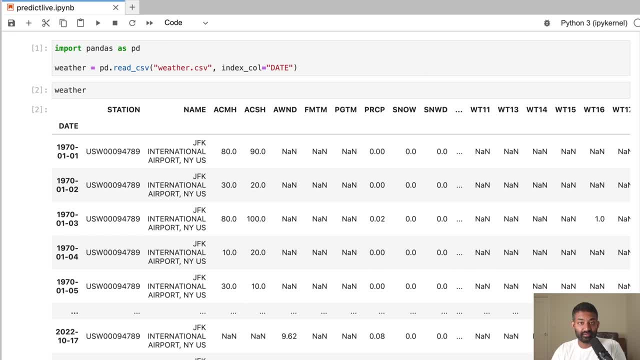 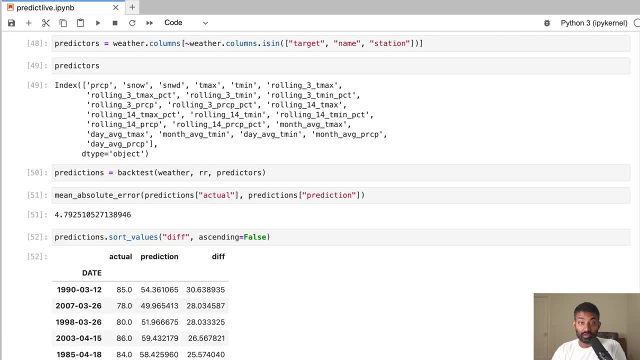 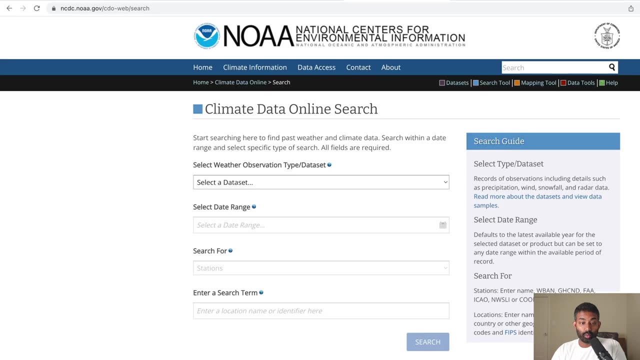 actually download a weather dataset from close to where you live and use that to make predictions. Second, we'll read in and clean the data. Third, we'll train a machine learning model to make historical and future predictions for our data. We'll download our data from NOAA, a US government. 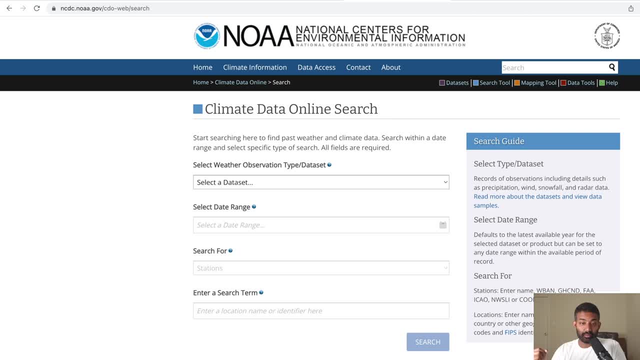 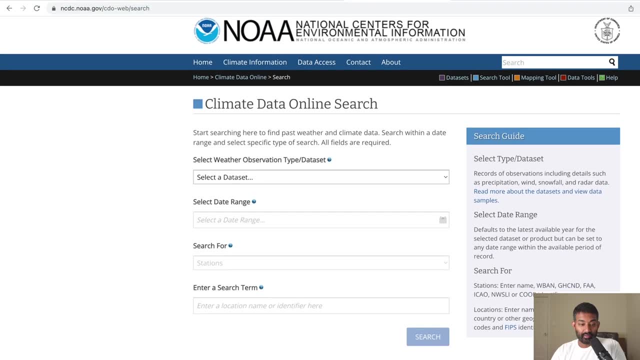 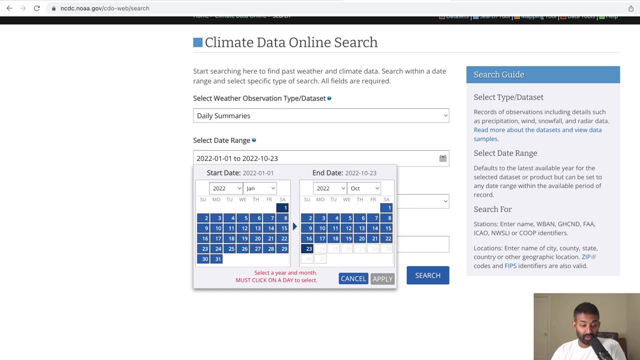 agency that actually forecasts the weather in a lot of places around the world, So they have great weather data. First we're going to go to this page, Then we're going to select Daily Summaries. Then we're going to select the date range of the data that we want. So we're going to pick 1970,. 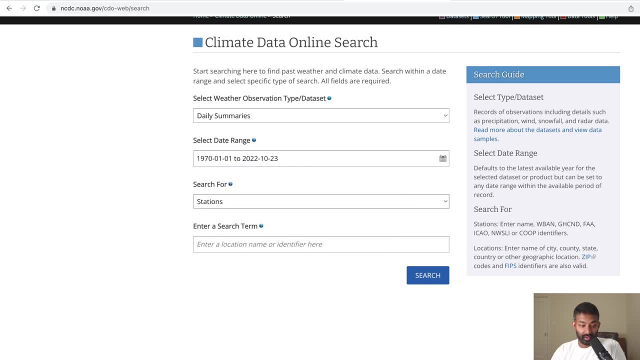 January 1st to the current date. We'll search for stations And what you can do is enter in the closest airport to you. So this actually has data for a lot of international airports too. So feel free to try the one near you. I'm going to try JFK airport. 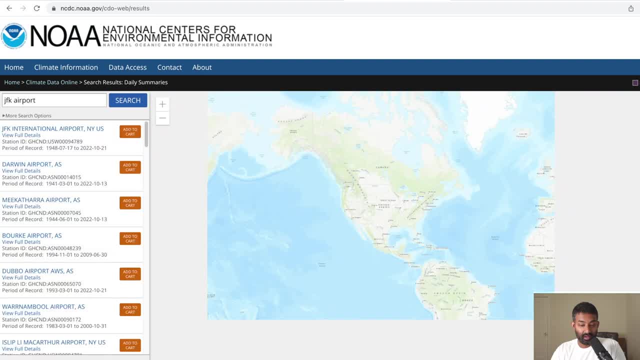 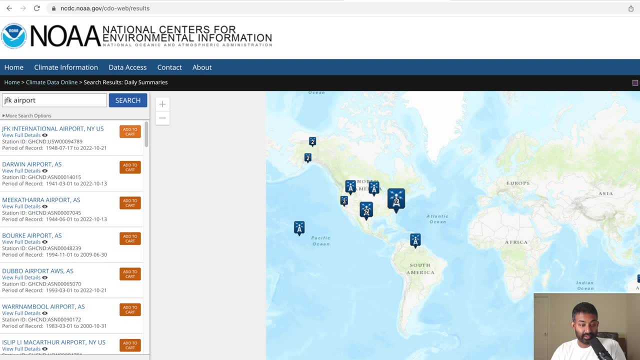 which is one of the main airports in New York City. Then you should come to this map view And on the left you'll want to just select the airport closest to you. I'm going to select JFK and click Add to Cart. Then, all the way over here at the right, you can actually go into your cart and view all items.